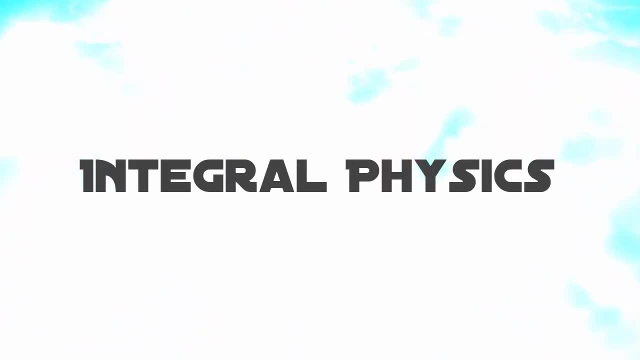 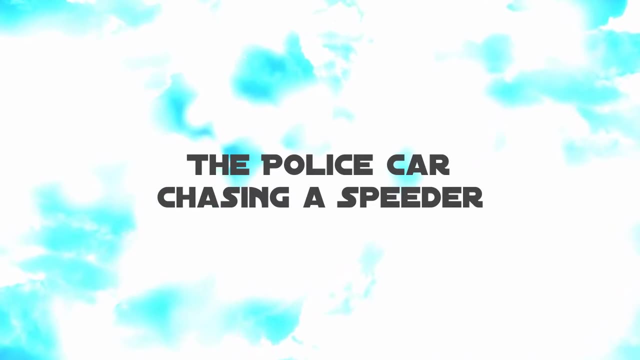 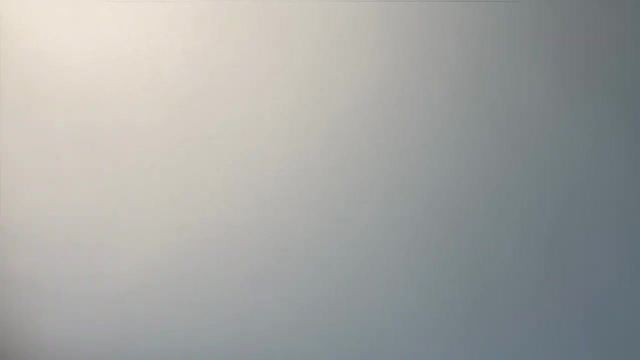 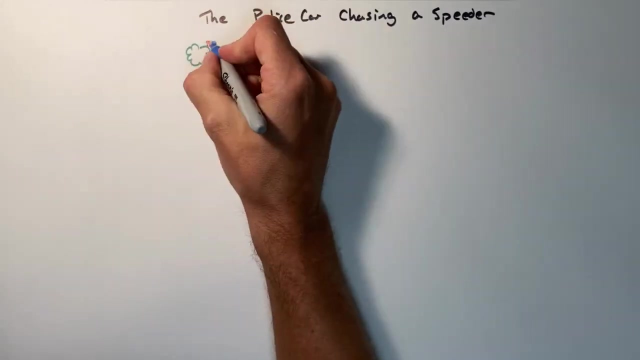 Okay, what we're dealing with now is the police car chasing a speeder problem. This problem is exactly what it sounds like. This is a police car hiding behind a bush. Now this police car sitting on this side of the road is looking down the road for speeders. 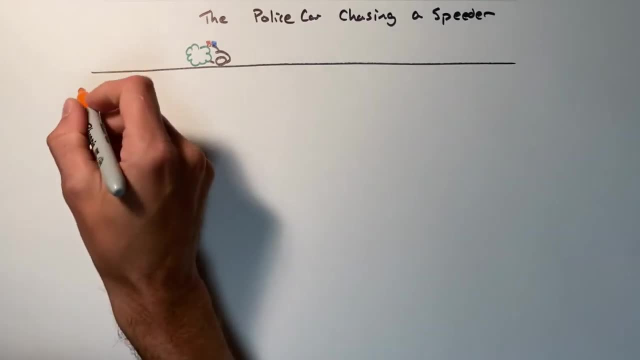 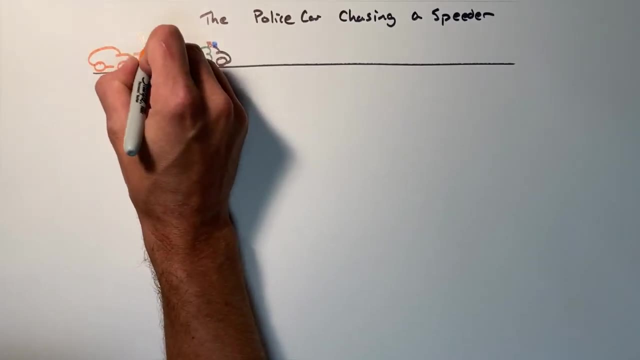 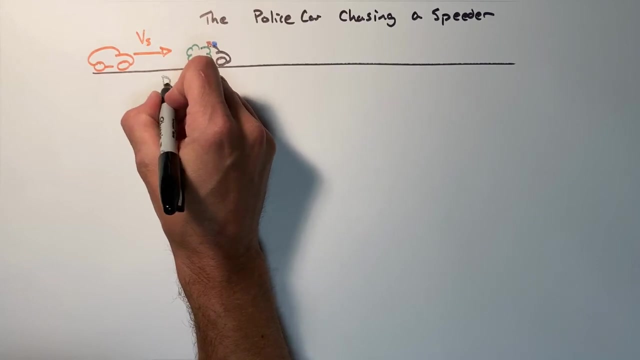 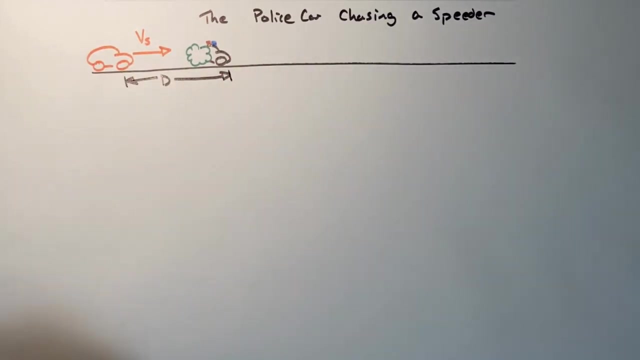 and so as the speeder approaches at some velocity V of the speeder, this police car is gonna see this guy coming and when he's some distance D down the road before he gets to the police car, the police car is gonna pull out. 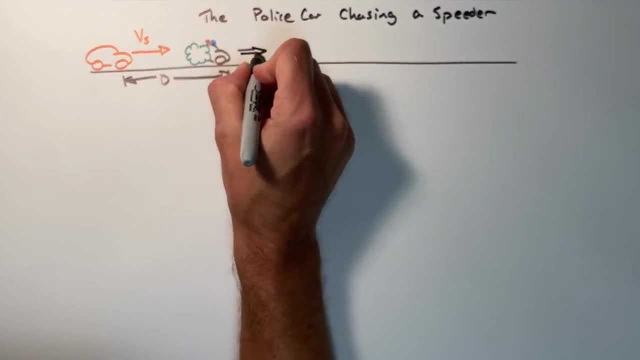 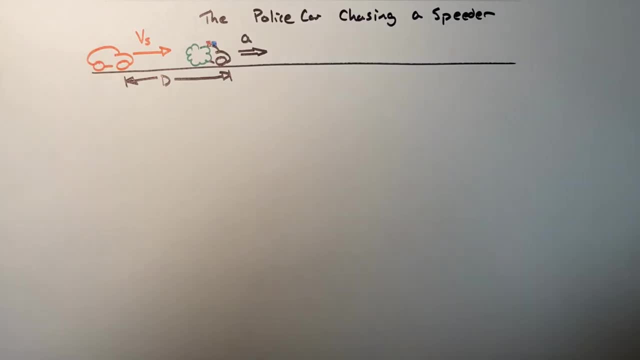 when the police car is going to in fact catch the speeder. So we're looking for time. how long that's going to take? Ultimately, what we want to do is we want to find the time when their positions of these two vehicles are the same. 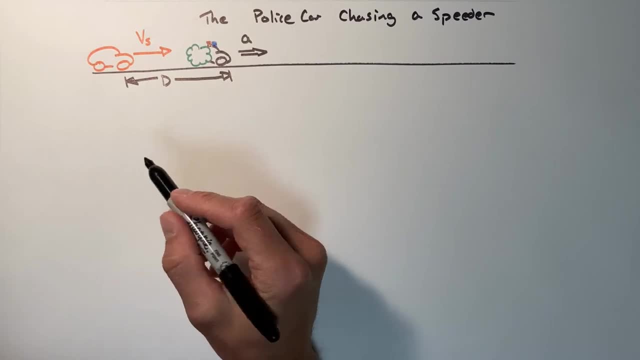 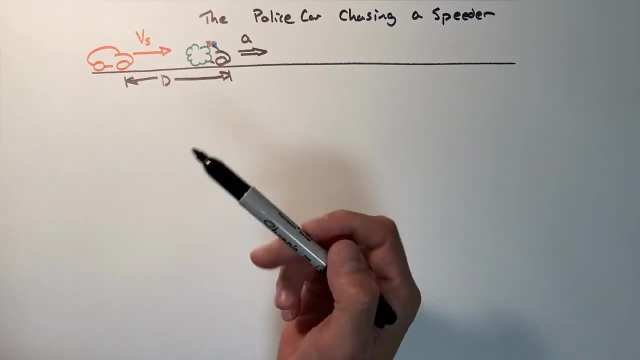 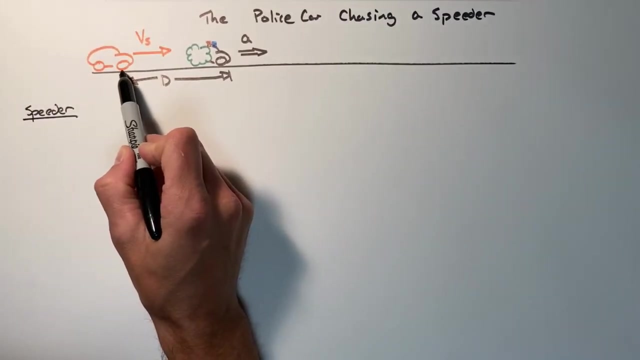 That's going to be when the police car catches the speeder. So we're going to use the kinematic equations and we're going to apply those equations to each individual car. So first let's look at the speeder. The speeder starts back here. 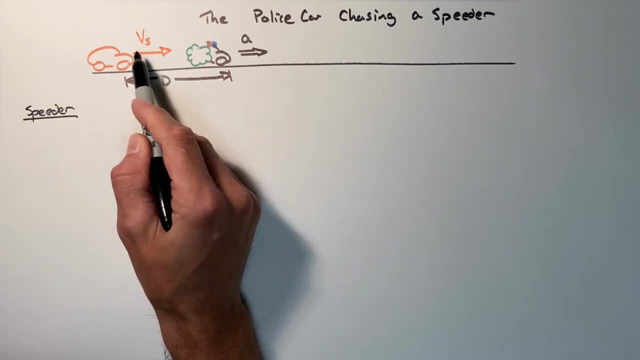 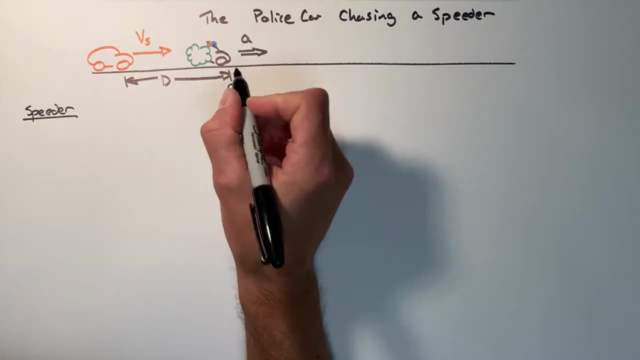 Let's travel along at some constant velocity Vs And we have to choose where to say: the origin is in this problem or a position of zero. I'm going to choose to say where the police car starts is a position of zero. You could just as easily say the position over here is zero. 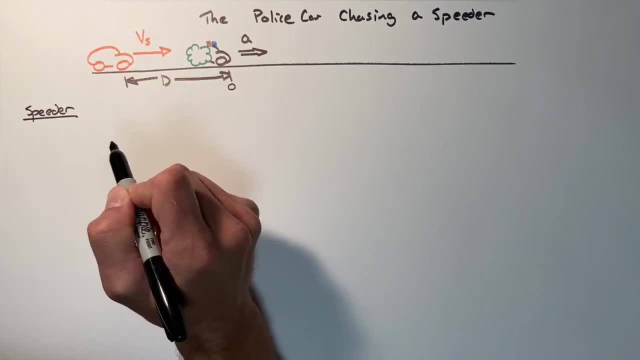 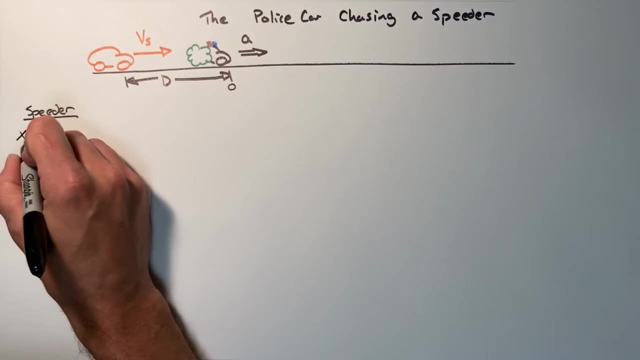 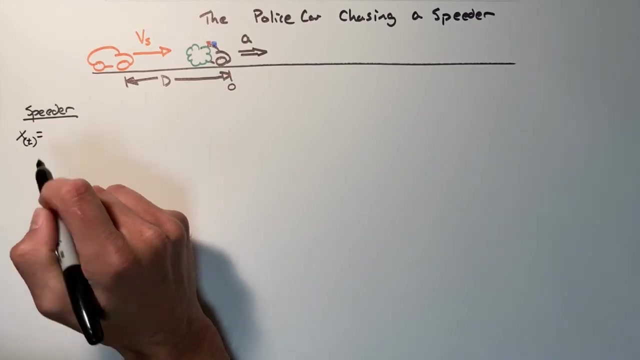 And we'll talk about How that will change things. if you chose to make this zero, The speeder is going to have some position as a function of time given by the position equation in the kinematics, So his initial position is going to be negative. d. 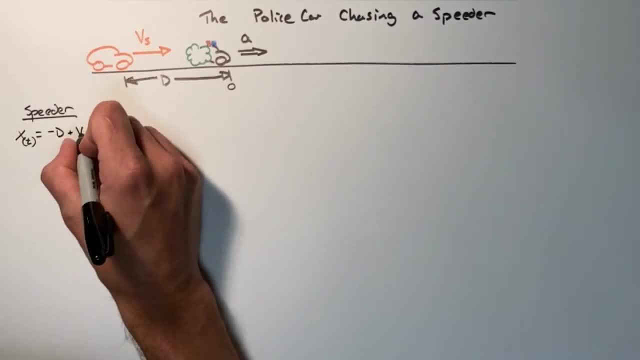 The velocity is Vs, So we're going to have a Vst for position. Now there is no acceleration. The speeder is moving at a constant velocity, So we're going to have plus one half times zero t squared, And you can see this term is zero. 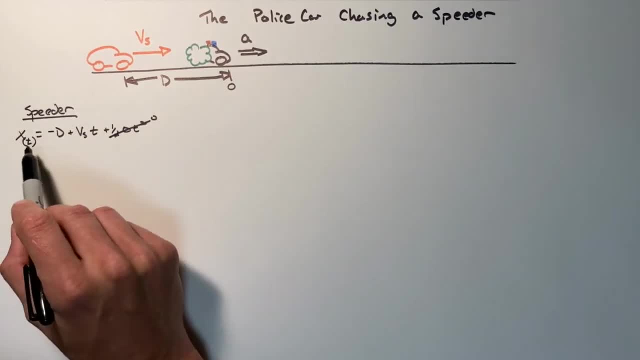 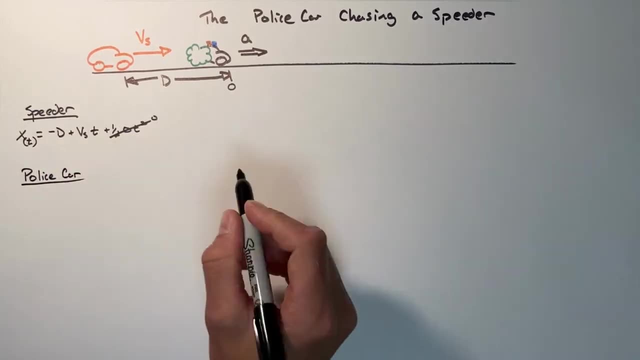 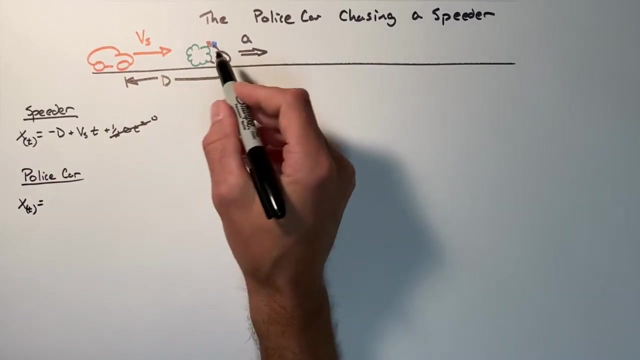 So we have this function for the position versus time of the speeder. Now let's do the same thing for the police car. We're going to use the same kinematic equation again, And this time we're going to apply that equation to: 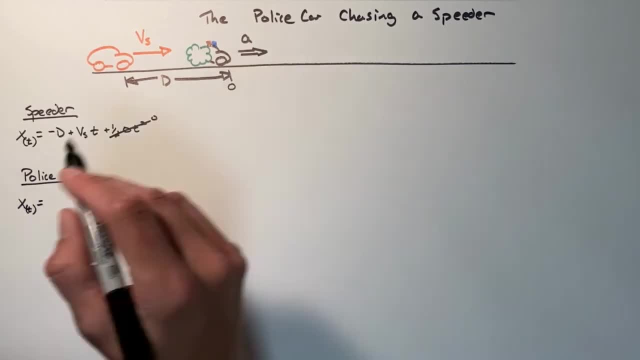 The police car. Now, the initial position of the police car is zero. The initial velocity of the police car is zero. Remember, he's starting at rest. He's hiding behind a bush shooting radar at speeders coming down the road. So we're going to have: Vi is zero times t. 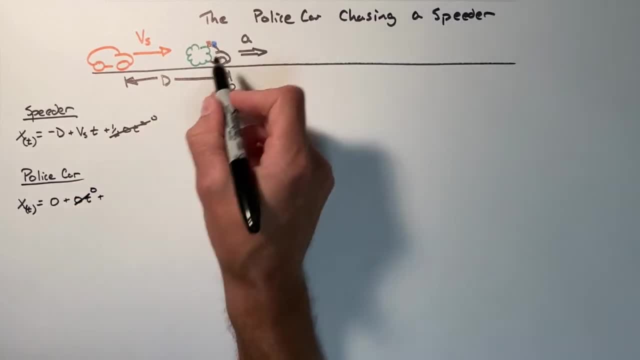 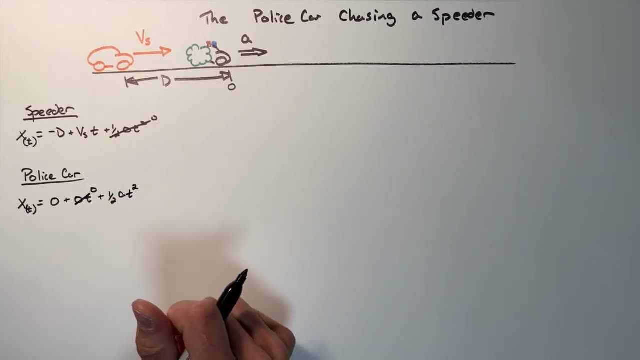 So that term is going to be zero. Plus we're going to have one half times the acceleration of the police car, Multiplied by time squared. Now realize when these two vehicles are at the same position. These two equations are going to be equal. 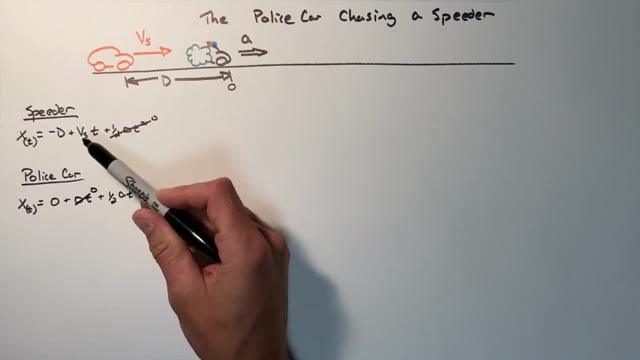 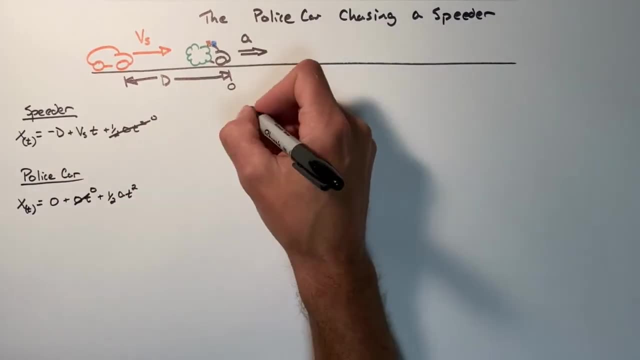 So the whole point of this problem is to solve for when or at what point in time The two vehicles are at the same position. So let's take these two equations and set them equal to each other. I'm going to say the position of the speeder needs to equal the position of the police car. 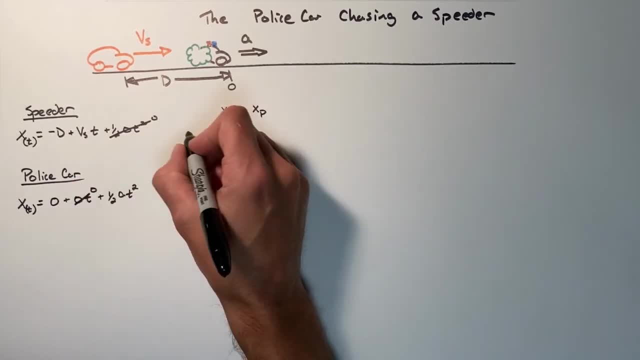 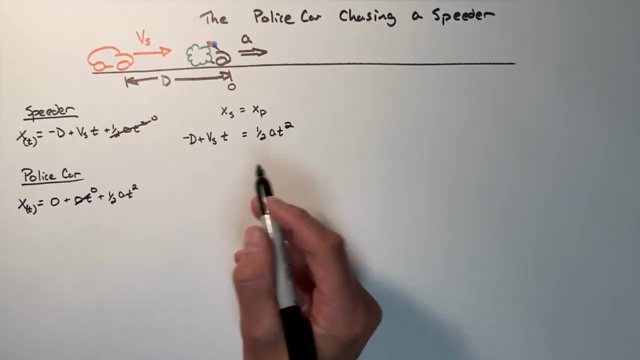 So I'll substitute in these two functions over here Now to solve for time, we simply need to use the quadratic equation. So we'll rearrange this to put this in a little bit more familiar order And you'll see, here we have this function here. 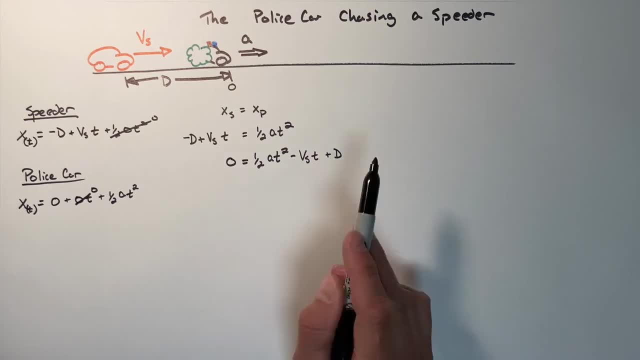 We're going to use the quadratic equation to solve this, And what's important to realize Is we have our standard terms that we put in the quadratic equation- A, B and C. So we'll write out the quadratic equation Subbing in these necessary terms. 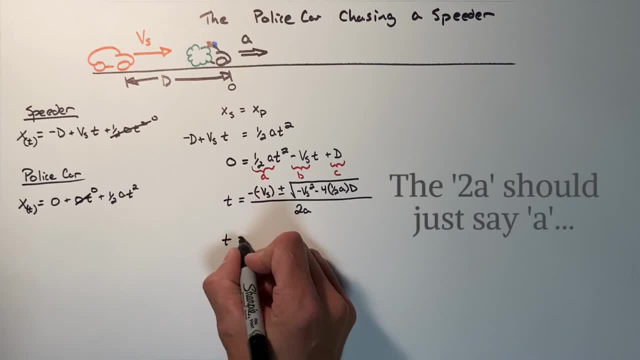 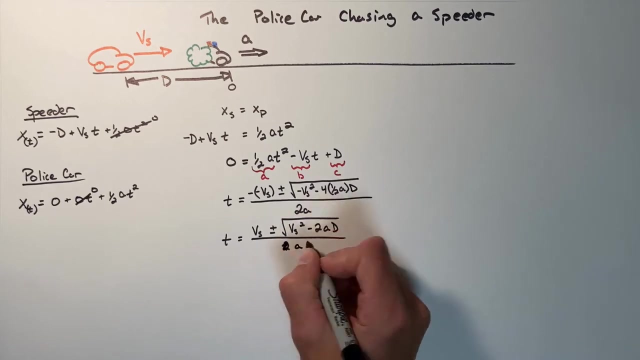 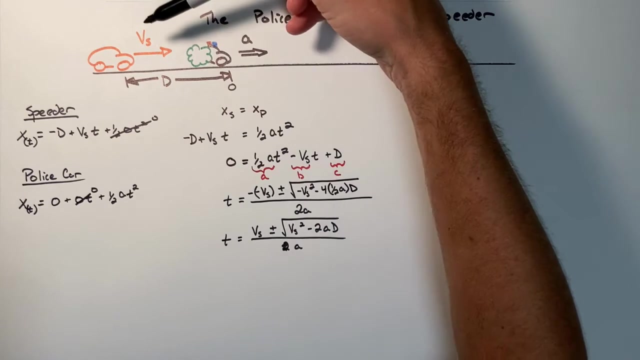 And then we'll clean this up a little bit, Subbing in, Subbing in. we have this function here. It looks like we have a result. We have a function for time where, if we knew the velocity, the acceleration and the distance between these two vehicles, we could 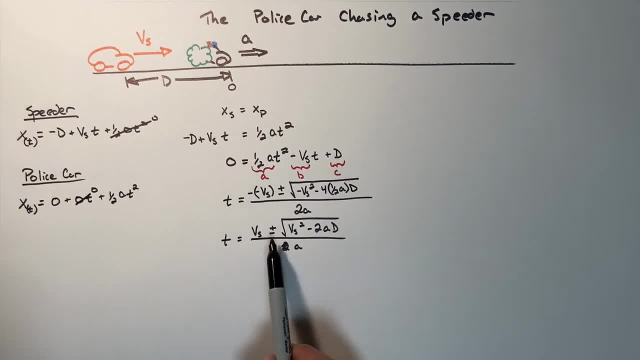 solve for the time. But there's a catch here, And the catch is right here. The quadratic equation always yields two results. In this case, there's a physical meaning to those two results, So let's talk about what those are. In order to understand what these two results mean, we need to look at 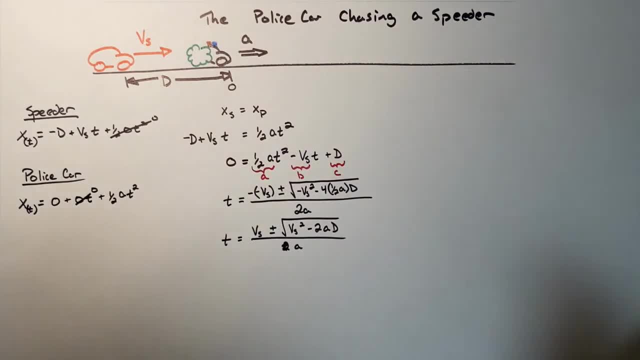 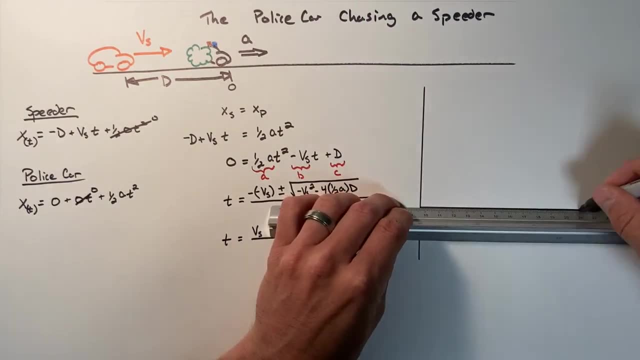 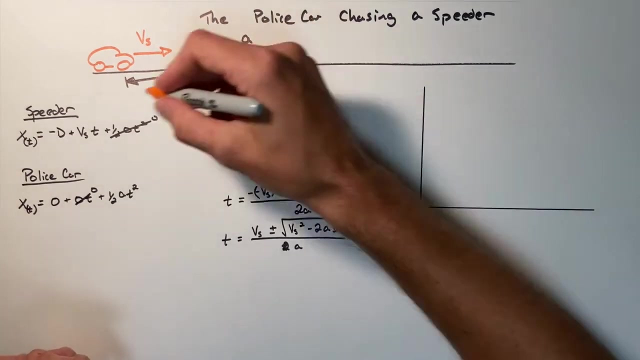 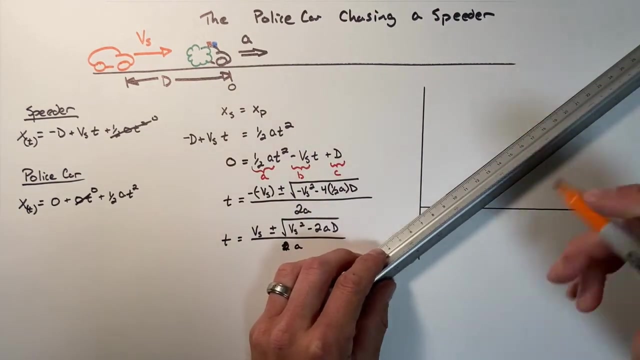 a graph showing the position and time for the two vehicles. Now, when we look at the speeder, the speeder starts at some position of negative d and travels forward at a constant speed. A constant speed on a position versus time is a constant speed on a position versus time. 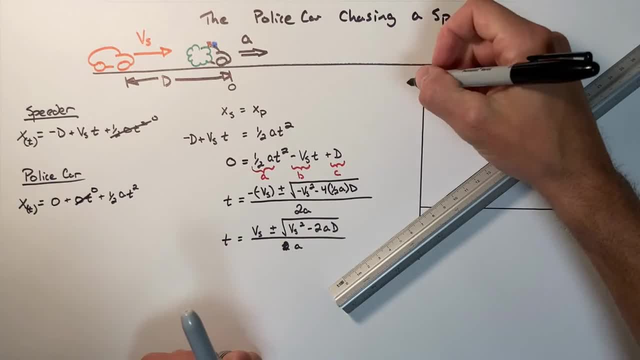 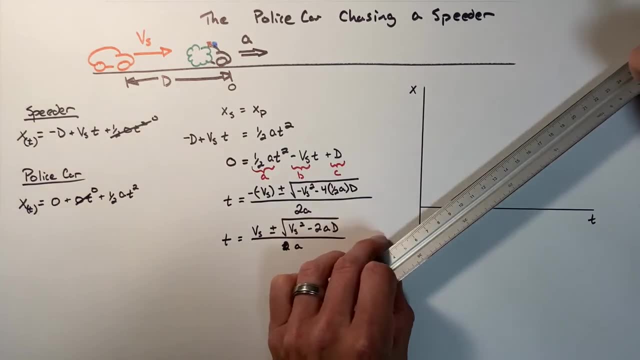 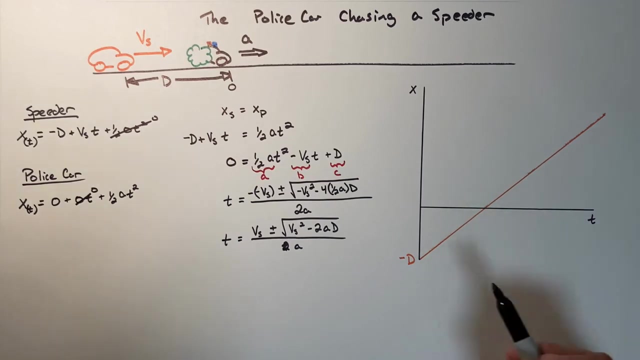 graph. it's going to look like a diagonal line, the police car. well, the police car is is starting at a position of zero and speeding up. so this police car is a function, is going to look a bit like a parabola and you'll notice there are, in fact, two points.